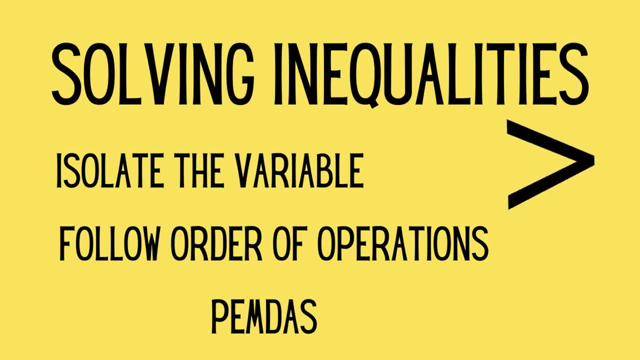 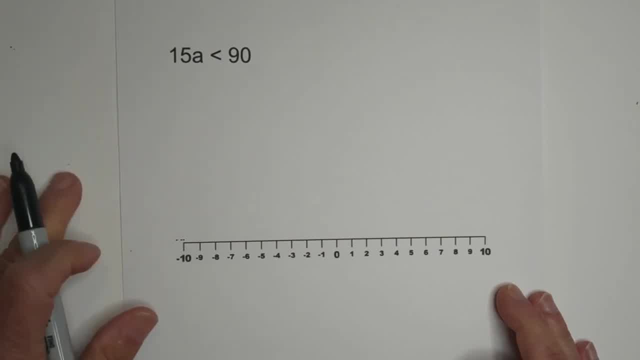 You must reverse the direction of the inequality sign. So let's get started with solving a couple of inequalities. Okay, so let's go ahead and solve this inequality and then graph it. So we need to get a by itself. So we will create an inverse operation. 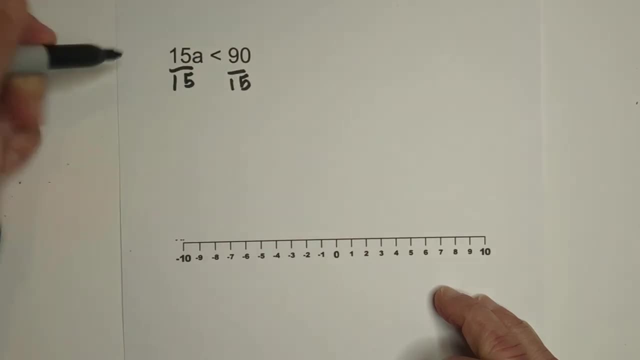 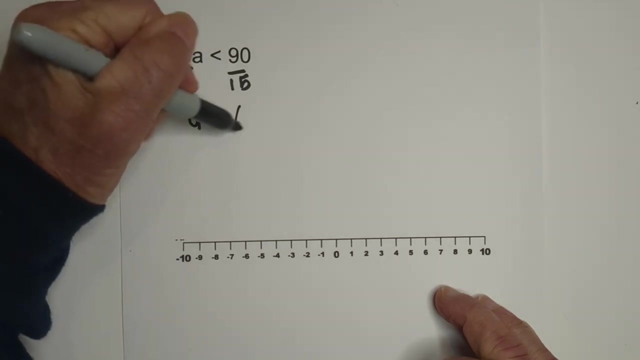 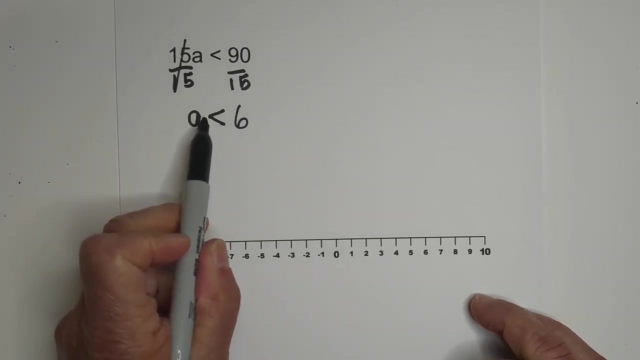 Divide both sides by 15.. When we do this, these cancel, bring down the a. So a is less than 90. divided by 15 is 6.. So now let's go ahead and graph this. And we know that since it is less than, so let's find 6, it's less than and it needs. 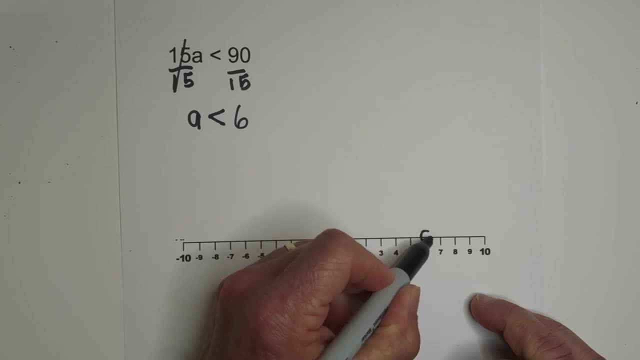 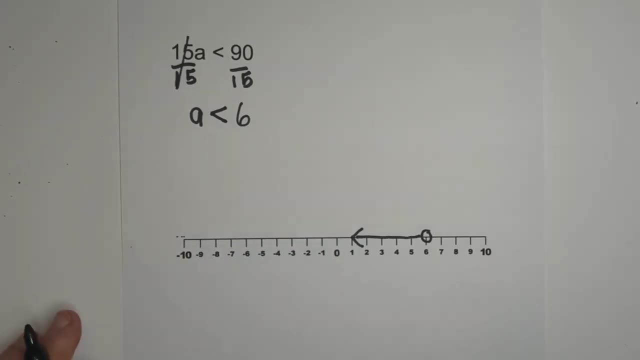 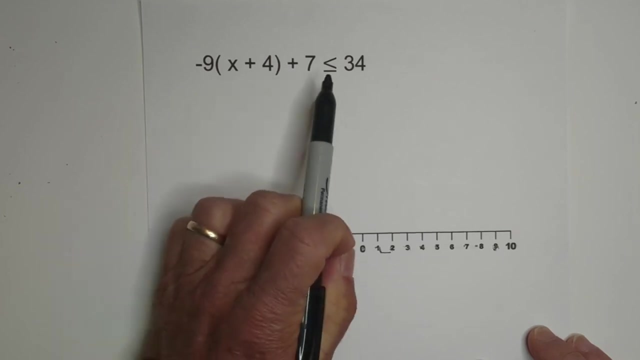 to be open, because it is not less than and equal to, so it will be less than 6.. So it will look like that on the number line. Okay now with this one, it introduces one thing: Whenever you divide by a negative number, you need to flip the inequality sign. 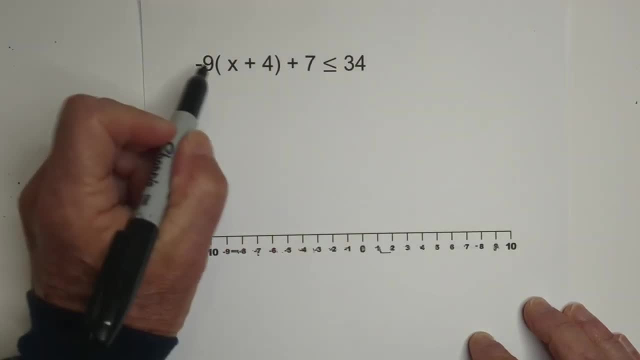 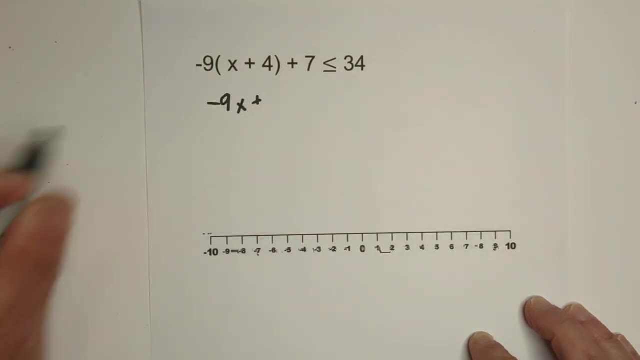 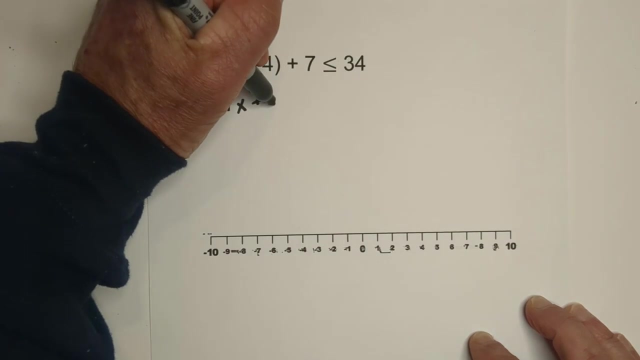 So let's work through it and see If we can't understand this. So let's first apply the distributive property 9 times x, So it will be negative 9x plus 9 times 4.. What is that? That will be 36, negative 36.. 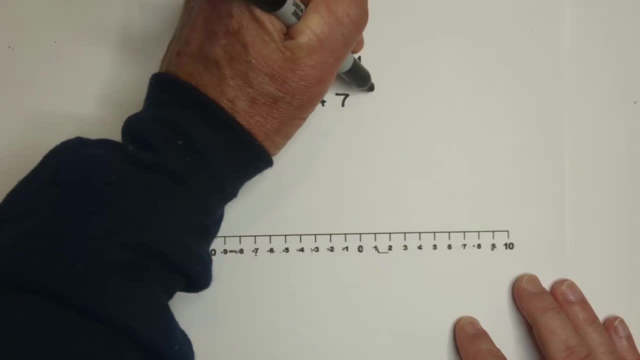 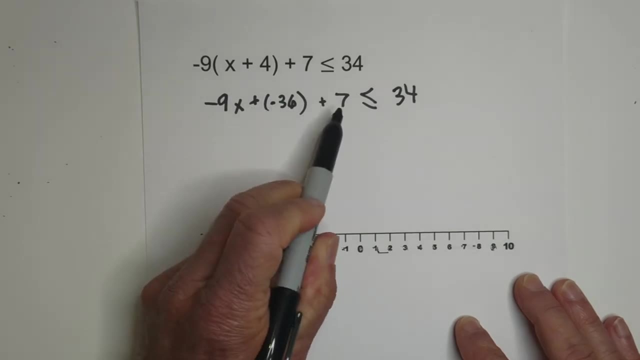 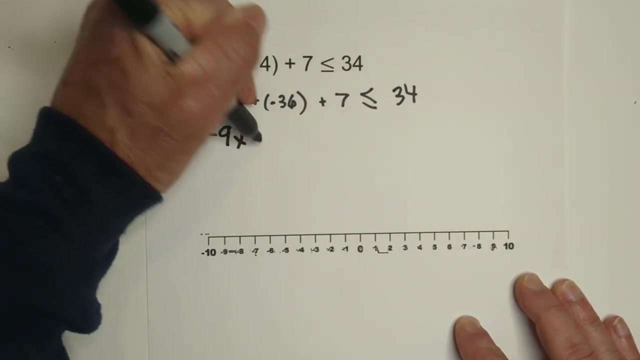 And then we have: plus 7 is less than equal to 34.. Now we can combine some like terms: negative 36 and positive 7. I'm going to bring this, I'm going to bring this down, and that will equal a negative 29.. 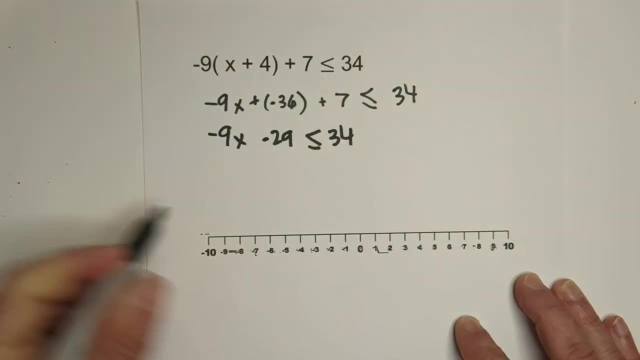 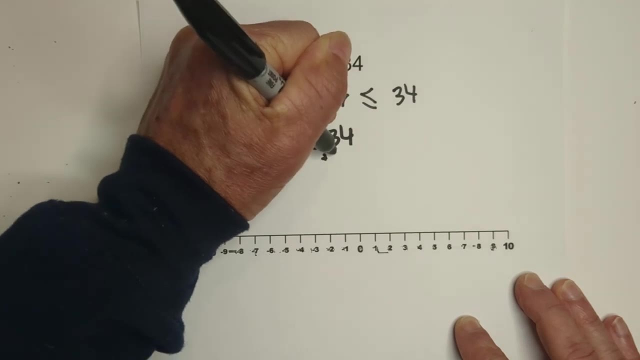 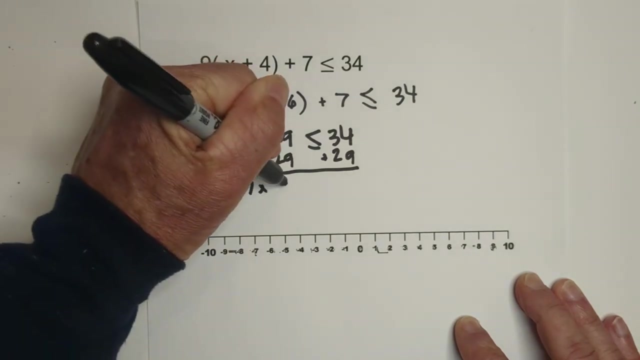 And then that is less than or equal to 34.. And so let's move the 29 to the other side by adding 29 to both sides. Okay, and so when we bring this down, we have negative 9x is less than or equal to these. 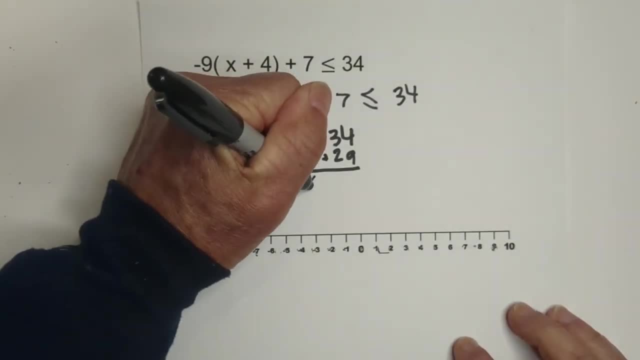 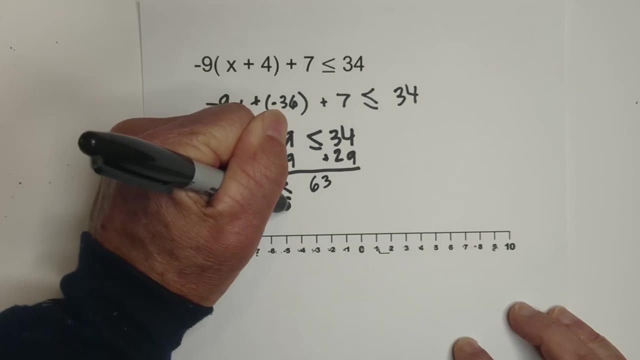 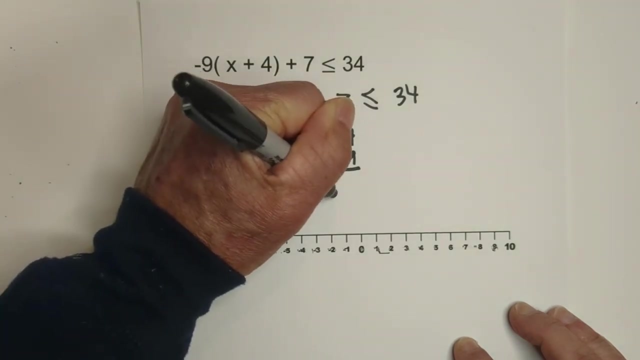 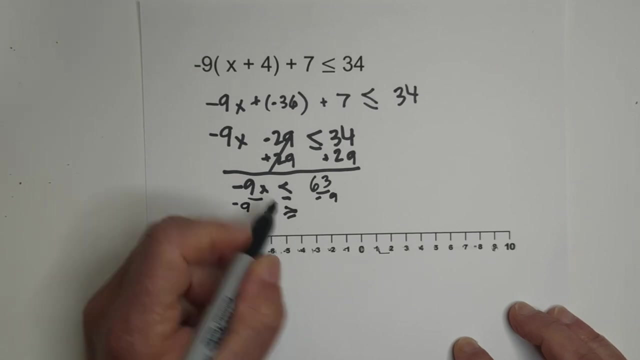 cancel. And this is 66. This is 63. And then we're going to divide through by negative 9.. And we need to flip the sign, okay. And so we're going to divide through by negative 9.. And so we have: x is less than or equal to 63. divided by negative, 9 becomes negative.